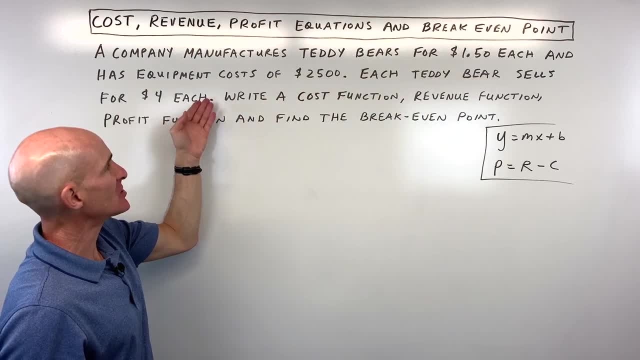 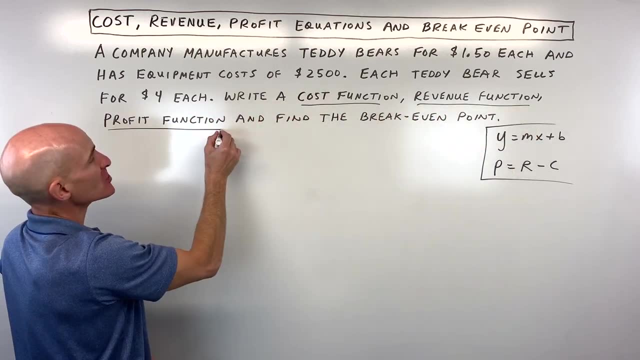 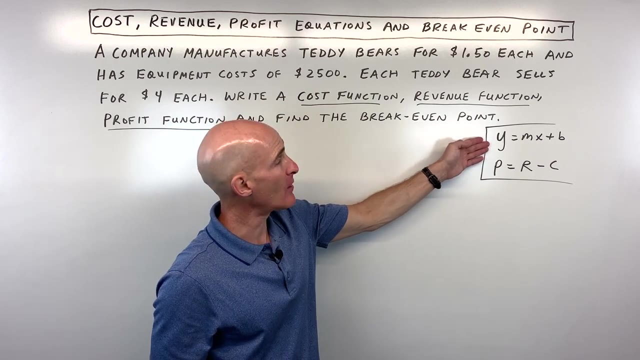 Each teddy bear sells for $4 each. Can you write a cost function, a revenue function, a profit function, and then can you find the break-even point. So let's take this one step at a time. Now, some equations that you might want to write down or memorize are the basic slope. 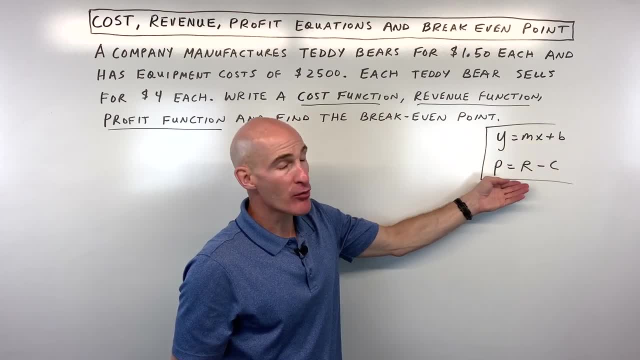 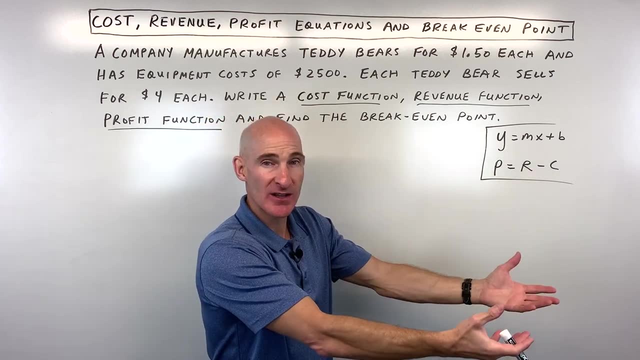 intercept form of the equation of a line as well as your profit equation, which, remember, profit is equal to the revenue, the money that you take in, minus the cost, the expenses or what you spend going out. So that difference is your leftover, which is your profit, right? So let's break this. 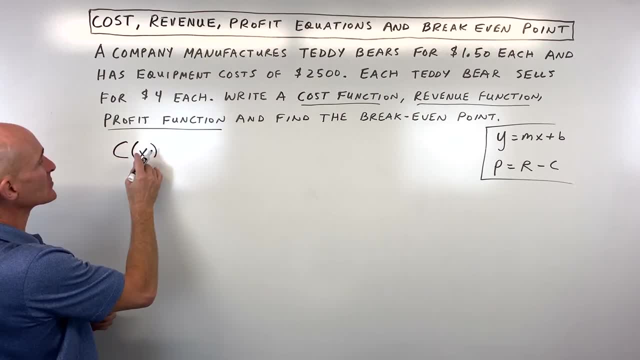 down one step at a time. So, for example, let's say you have a company that manufactures teddy bears. for the cost, let's say c of x, where x is the number of teddy bears sold, It's going to cost $1.50. 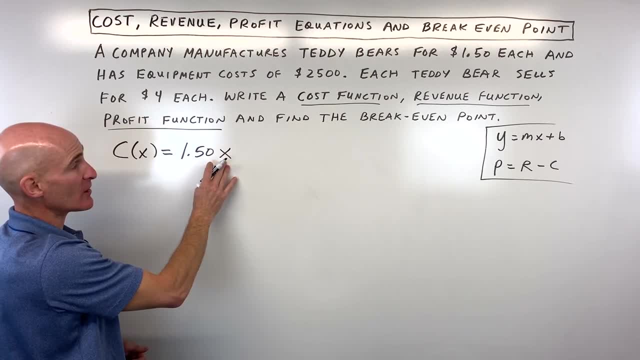 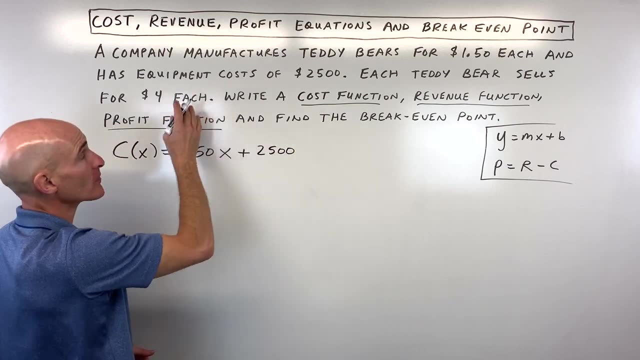 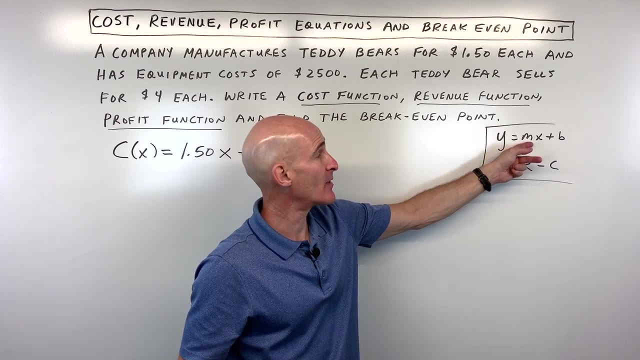 times x the number of teddy bears that you're making or manufacturing. plus it also costs you the initial expense of the $2,500 for the equipment. So remember, when you think of the slope or the m-value, that's like the rate, like how much it costs per teddy bear to make, whereas the b 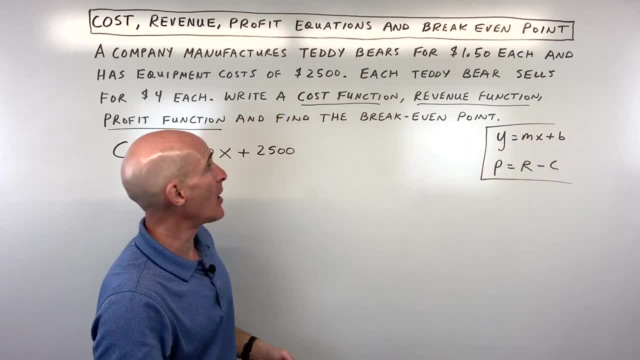 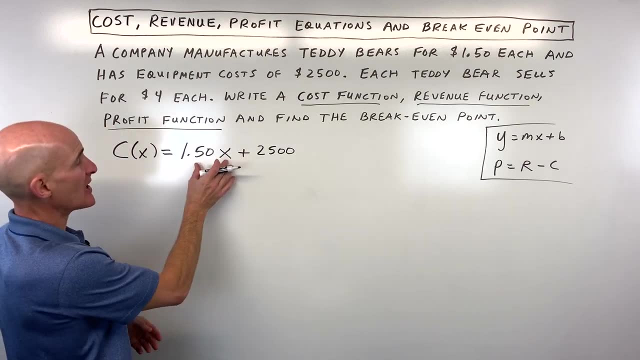 that's our y-intercept, or our initial condition, or a starting amount, and these were our starting expenses. the $2,500, that's just a fixed or constant cost, Whereas this is going to increase as you make more and more teddy bears. So that's our cost function. Now the revenue function, that's how much money that you're. 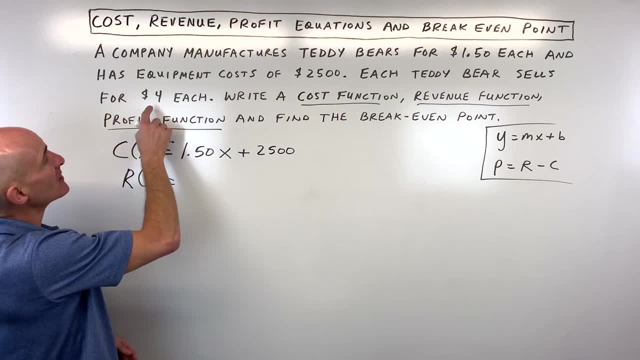 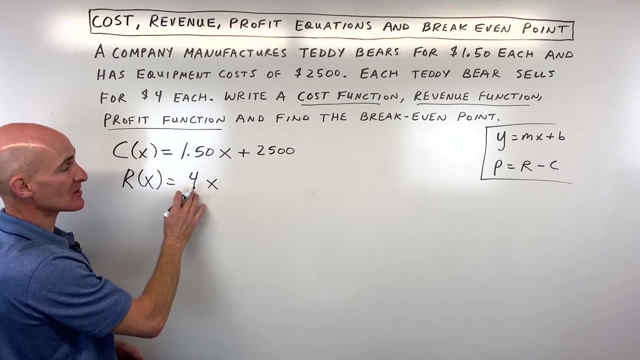 making right when you sell these teddy bears and they're saying that we sell them for four dollars each. So it's going to be four dollars times the number of teddy bears that you sell. If you sell ten, it's going to be four times ten forty dollars that you're taking in And then our 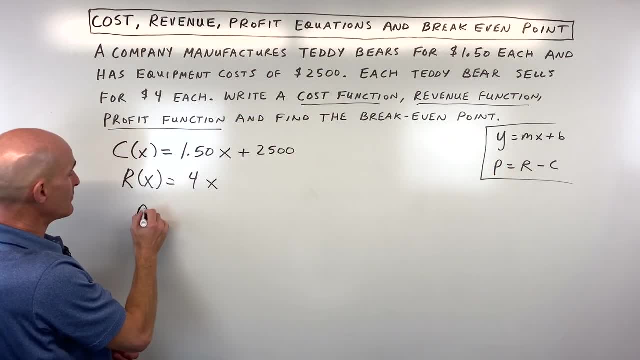 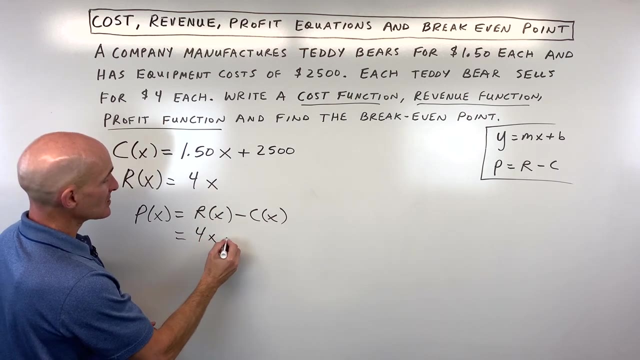 profit is again, like we said, the difference. so we're going to say p of x is equal to r of x, our revenue minus our expenses or our costs. Now, one mistake that students sometimes make is they forget to use parentheses. so our revenue is 4x, our cost is this whole thing. so let's put it in parentheses. 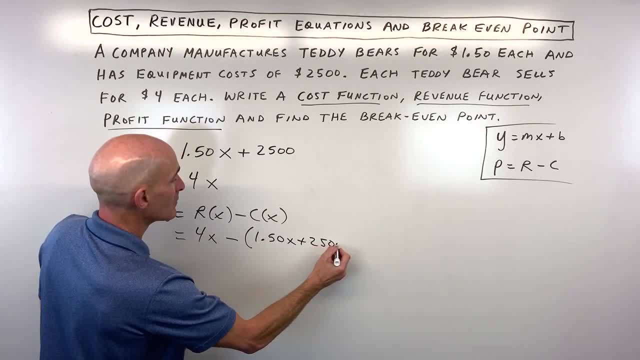 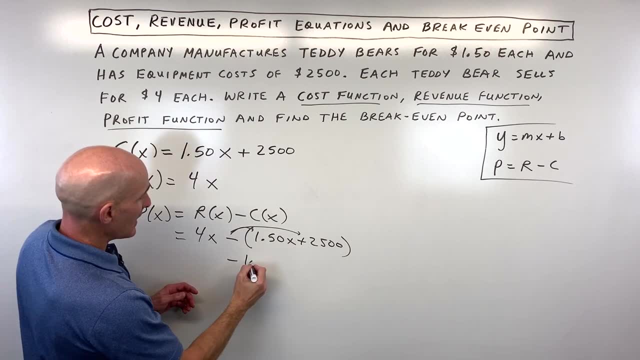 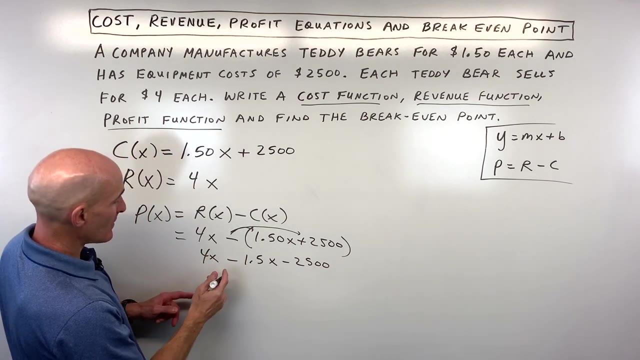 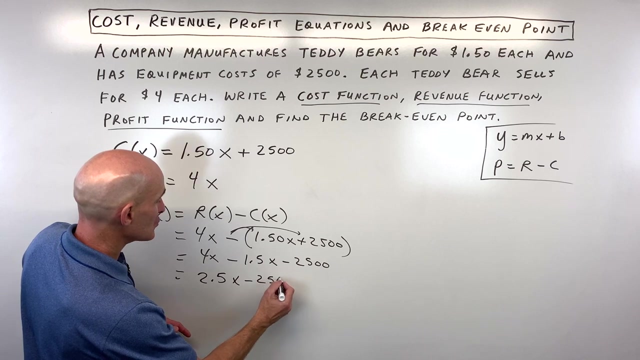 let's treat it like a group. and now what we're going to do is we're just going to distribute this negative one into the parentheses, which is going to make this a negative 1.5x minus 2500, and if we combine like terms, let's see 4x minus 1.5x is 2.5x minus 2500 and that's our profit. 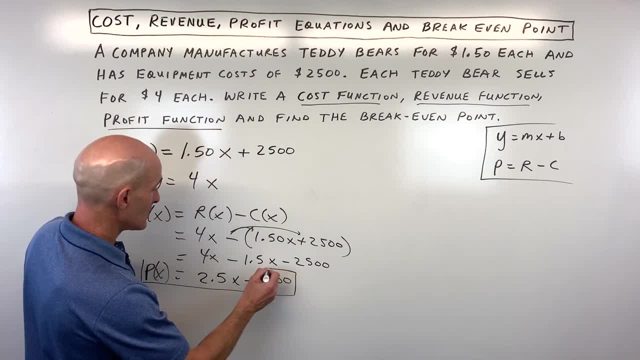 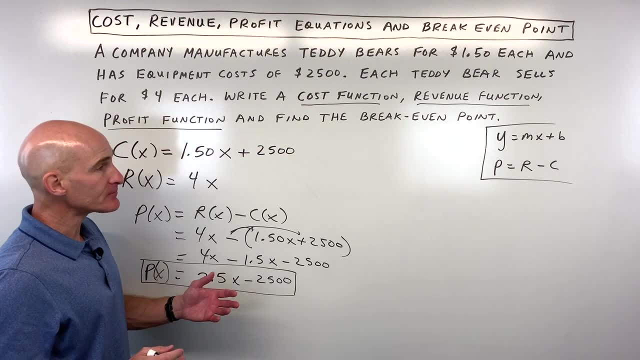 okay, as a function of the number of teddy bears. okay, x. Now to find the break-even point. what is the break-even point? It's the number of teddy bears. So we're going to find the number of teddy bears. So what is the break-even? Well, basically, the break-even is when the amount of money that 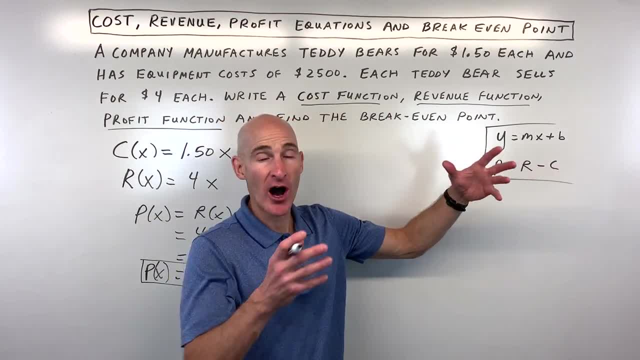 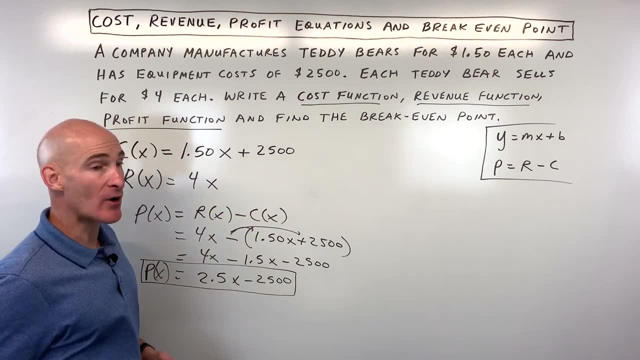 you've taken in is the exact same amount as the cost for your expenses going out. so, really, that profit at that break-even point is going to be zero, after which then you start to become profitable. so what we're going to do is we're going to set this p of x here equal to zero, and we're going 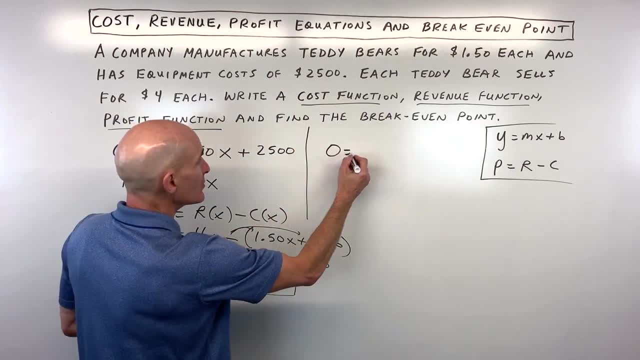 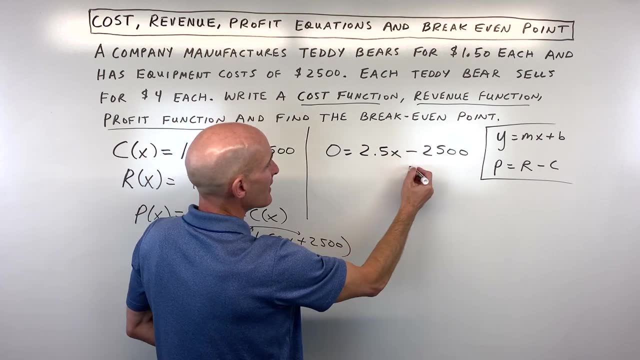 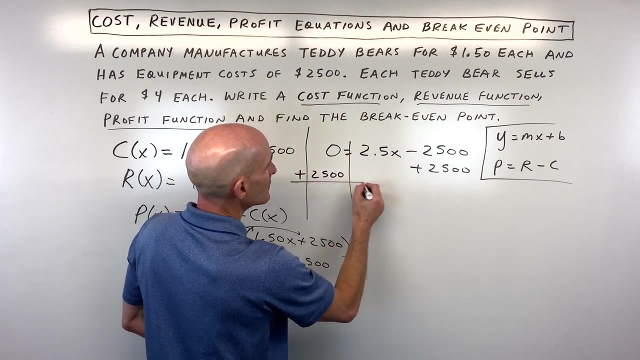 to solve. so let's go ahead and do that. we've got zero equals 2.5x minus 2500.. I'm going to add the 2500 to both sides to get the variable by itself, okay, and so you can see we have 2500 is equal to. 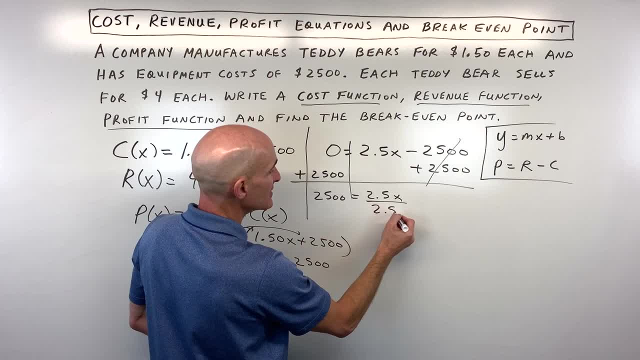 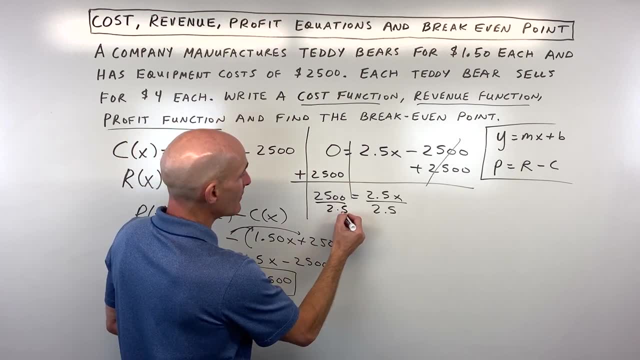 2.5x. We're trying to solve for the number of teddy bears that need to be sold and made in order to make a profit of zero. that's our break-even. so divide both sides by 2.5 and 2500 divided by 2.5. 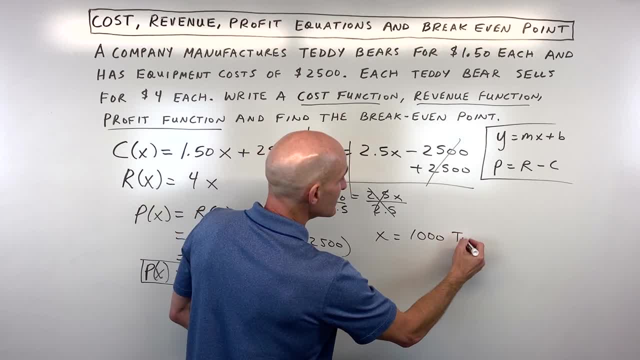 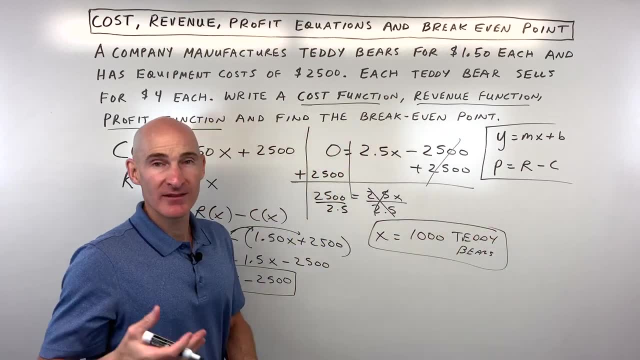 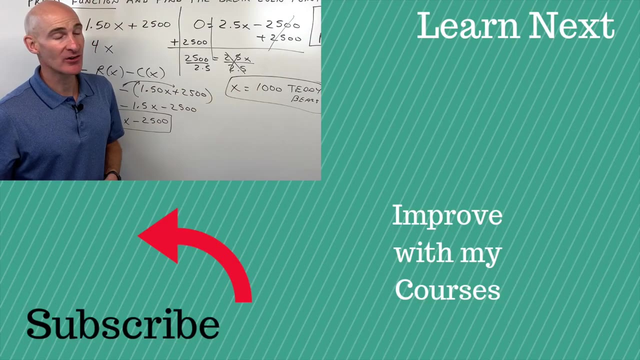 is equal to 1000.. Teddy bears, and that would be your break-even point. so once you sell a thousand and one, then you're into the black as far as being profitable, and if you sell less than this, you're in the red, whereas you're still in the you know. basically, you haven't made money yet you haven't broken. 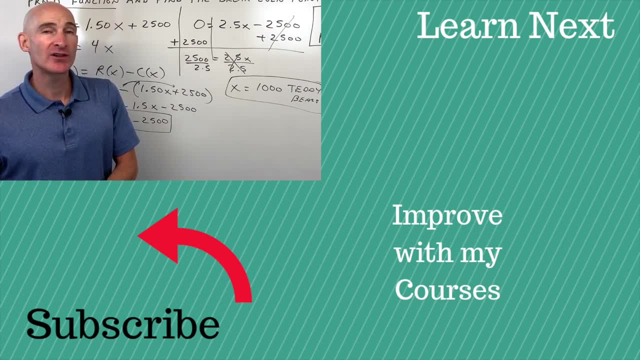 even so, great job. If you want to see another example where I talk about profit, revenue, cost, I'll put another video right there. follow me over to that video and try maybe some of those problems on your own. I'll see you in that video.